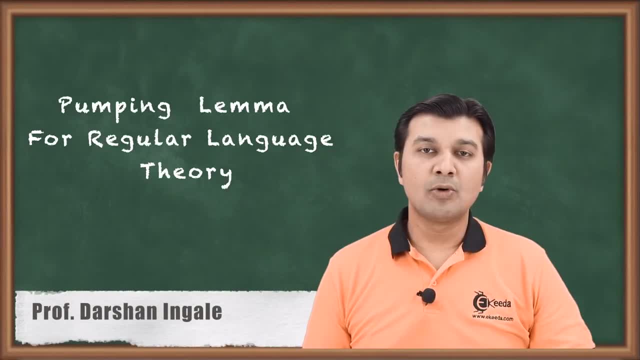 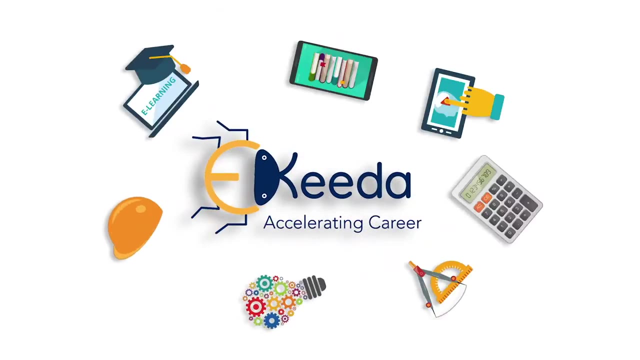 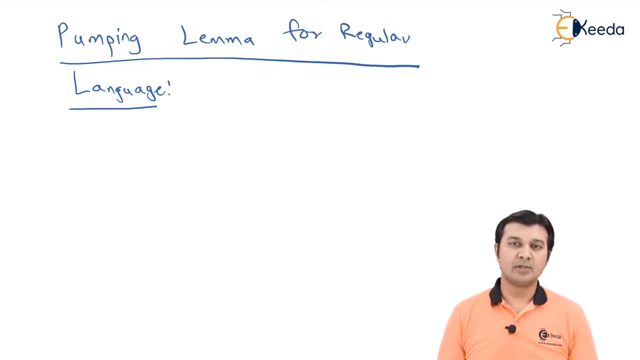 Hello friends, welcome to the next chapter. Over here we are going to understand the concept of pumping lemma. Honestly speaking, this is not a chapter. This is a subtopic itself and important short note which is asked in the exam. So now, pumping lemma for regular language. First of all, we know what is a regular language, right? So we also know why is a regular language insufficient for not solving some of the problems. 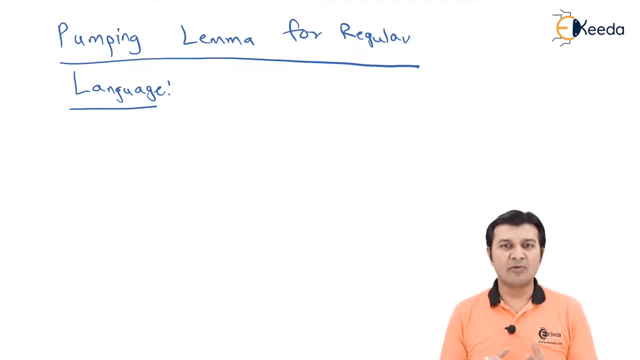 That is the reason we moved from finite state machine or finite automata to push down automata and further to Turing machine. So now pumping lemma is basically a kind of theory to prove that our language is not regular. Now let us understand. what do you understand from this? 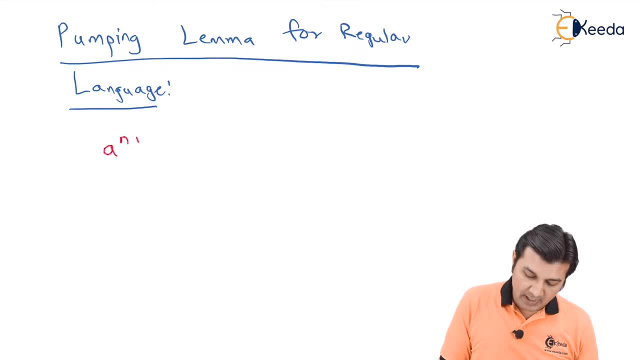 Let us say you have a problem for solving A raised to N, B raised to N, Where I have given N's value is going to be between 0 to 4.. And if I say, please design a finite automata for the same. 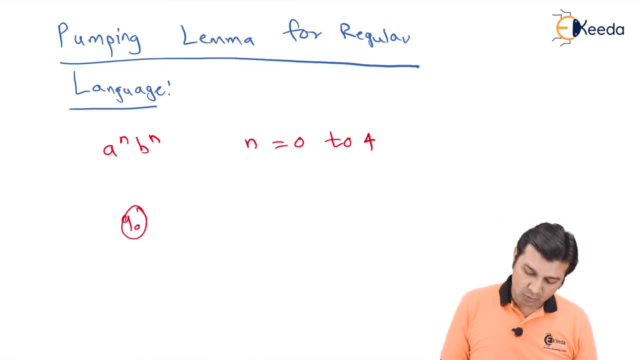 So you may say, you may have a state like: Let us say Q 0.. On getting A goes to Q 1.. On getting one more A goes to Q 2.. On getting one more A goes to Q 3, and this on getting a B comes over here. On getting B over here. 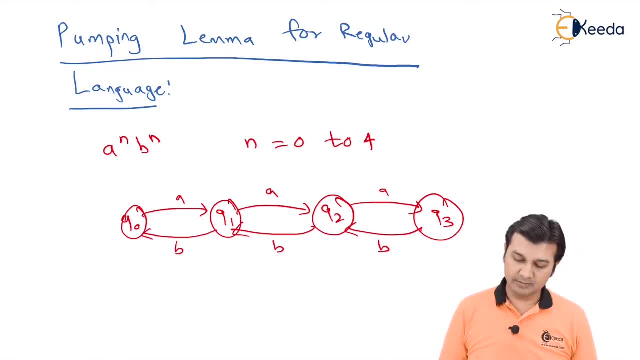 On getting a B over here. So what did we see that the number of A's and 3 number of B's can satisfy. So let us add one more, Q 4, over here, Where, on getting an A, it comes over here. 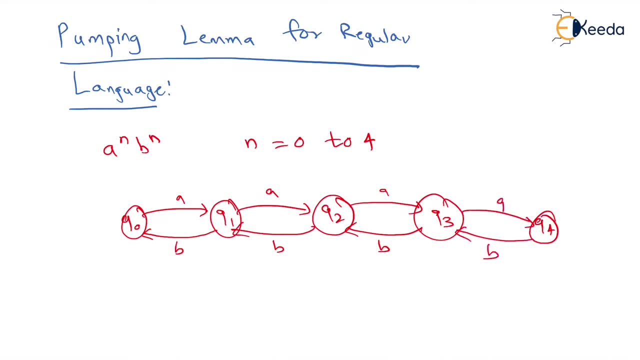 There we go. So I will now glymph. Now let us see what I am going to do. So let us add a 엇 and let us say: I perform fx to fx here on a, b, it comes over here. so now, friends, when we start from q 0, we see that if i have 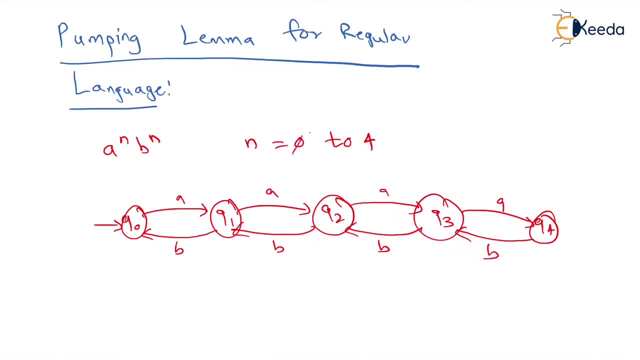 n's value is equal to. let's not consider 0, consider 1. so n's value would be 1. so that would generate the string a, b and is a b accepted, q 0 goes to q 1 on a, q 1 on b comes to q 0 and we. 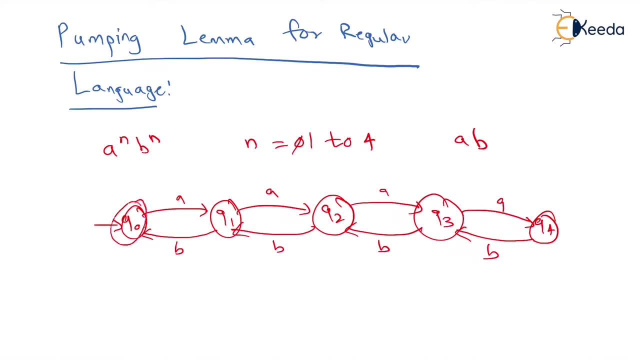 go to the final state. that's accepted. if we consider n's value as 2, the string is double a, double b, and that also is accepted. by going from q 0 to q 1, q 1 to q 2, q 2 to q 1, q 1, back to q 0. 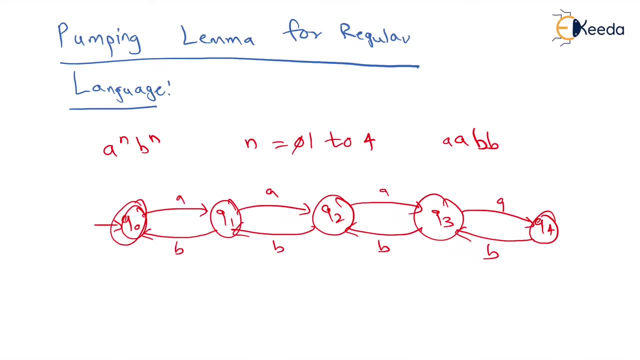 similarly, n is equal to 3, that is, 3 a's and 3 b's are also accepted. n is equal to 4, that is, 4 a's and 4 b's are also accepted. right, what if i say it has to be not for n? 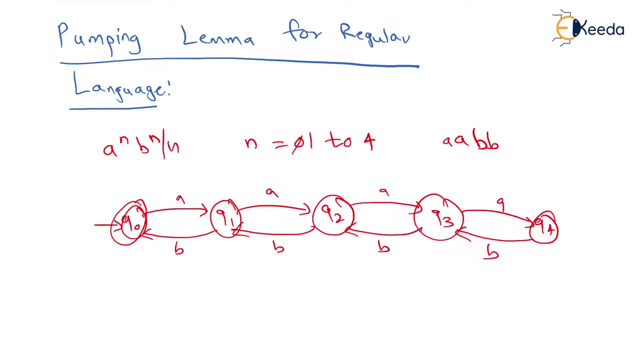 0 to 4 or n 1 to 4, but it has to be for n greater than equal to 1. so if this is the language, everyone might be coming on with the solution that let us keep on pushing the remaining a's over here and pushing the remaining b's over here, and this is going to satisfy. 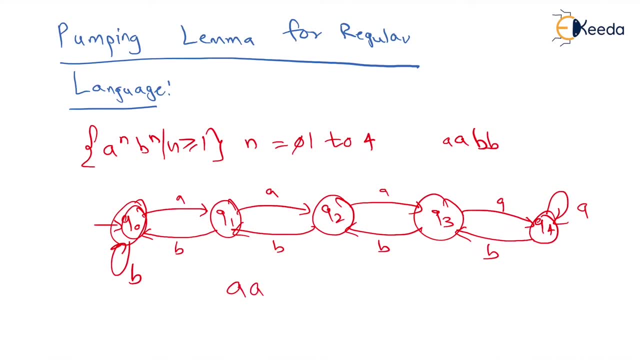 you can check. let us assume we have six a's, so we will be having six b's. so of this six a's, four a's would be utilized for going from q 0 to q 4, and the remaining a's would be in the cycle of q 4 itself. so two of the a's would be in q 4 itself. 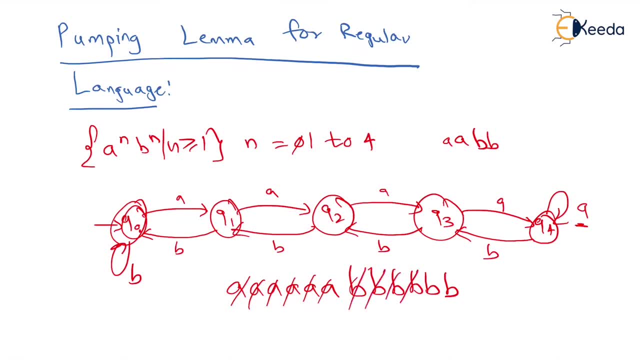 further this four b's would be utilized in coming back to q 0 and two of the b's will be utilized in q 0 cycle itself. and this machine is accepting for n greater than equal to one. but, friends, what if i have a input like a, a, a, a, a, just followed by four b's, or maybe more number of a's, and followed? 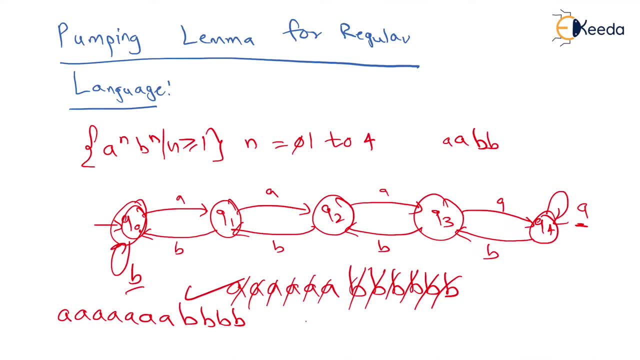 by this. so now over here. first and foremost thing, this particular thing is not of the form a raised to and b relation, because the number of n's of a are greater than number of n's in b. so this should not be accepted by the machine which we have designed. let's see whether this machine does not. 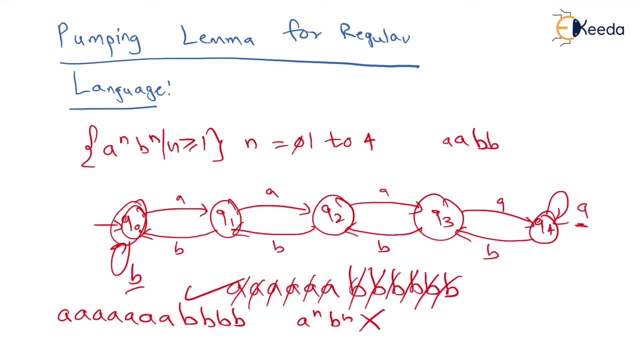 accept it. so for this first four a's, i go from q0 to q4. for the remaining three a's, my q4 is going to run in a cycle and take all these a's. then for the four b's, my q4 come backs to q0 and it is accepting. 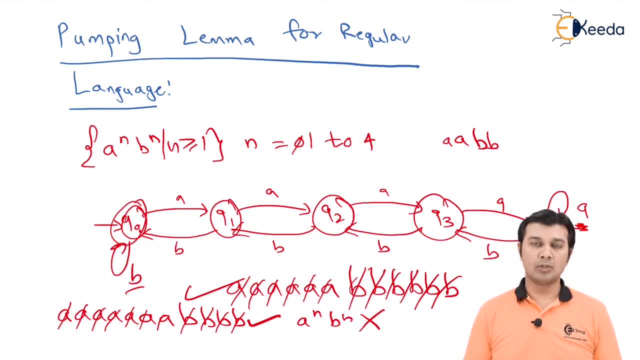 this input, which ideally it should not. so we have found a drawback over here that my regular language cannot be designed using the finite automata. so for such type of language or such type of problems which are not capable of being designed using finite automata, we have to go for the next machine which we have already studied, called as push down. 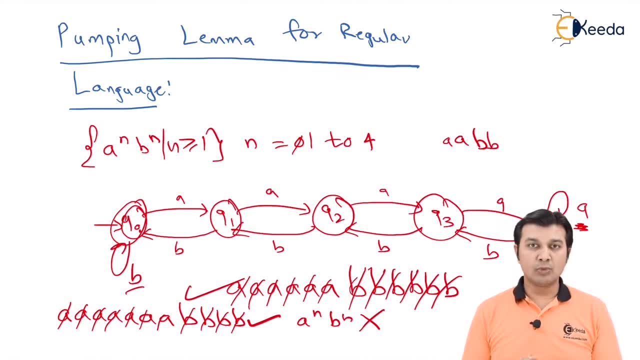 automata. so, friends, as i told you earlier, pumping lemma is basically a kind of theory which is going to prove that a language is not regular. therefore, it cannot be designed using finite automata. so that is what we are going to study over here. so let's understand some theoretical aspects of pumping lemma. the concept is actually very, very 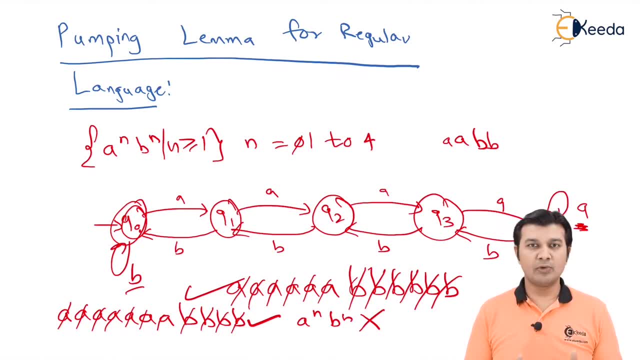 very simple, honestly speaking, if you keep your head a bit aside and understand it, because if you try to get into the deeper mathematics of it, you are going to waste a lot of time and energy over here. we have to be practical. it is simply going to be a five mark short note in the exam. 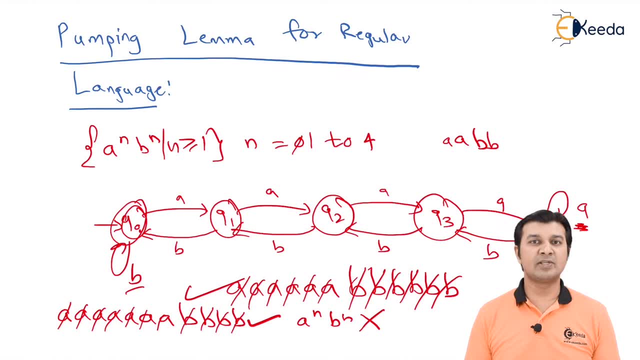 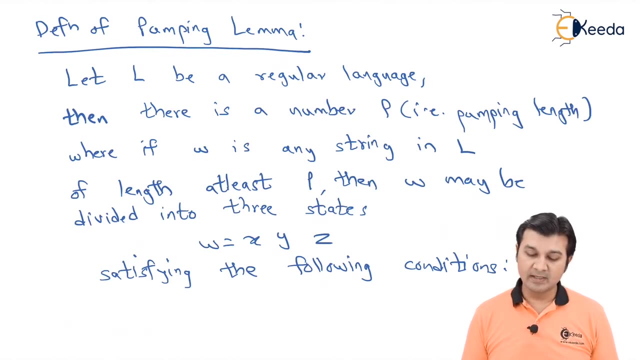 what is important i'll be focusing over here, and that itself has to be written in the exam. that's what we are going to study over here, so let's go ahead and start with the theory now. how do you define a pumping lemma? i say let l be a regular language. then there is going to 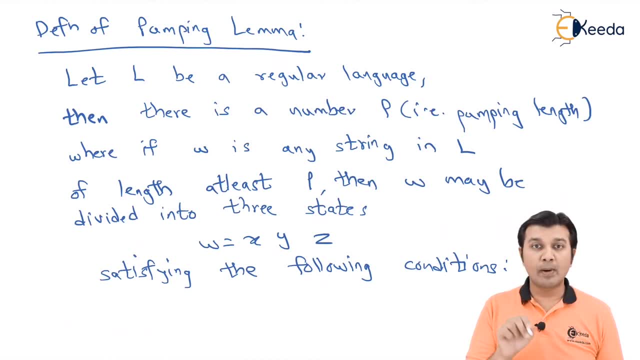 be a number called as p, which is called as pumping length. now, pumping length is going to be the cycle which we discussed over q4 and q0, so i'm going to keep on pumping more number of inputs in that particular state. so let l be a regular language then. 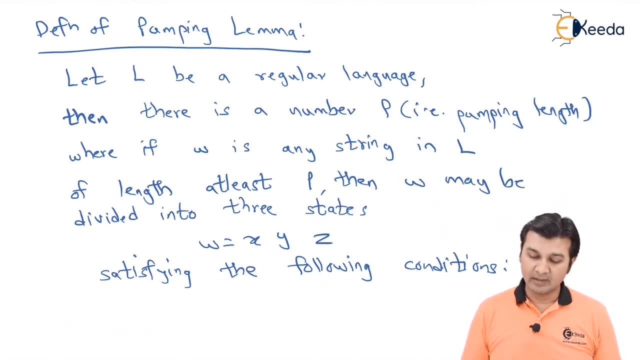 there is a number, p, that is pumping length, where if w is any string in that particular language of length at least equal to the pumping length, then w can be divided into three parts. w is equal to x, y, z, and these three parts have to compulsorily satisfy the below three conditions. 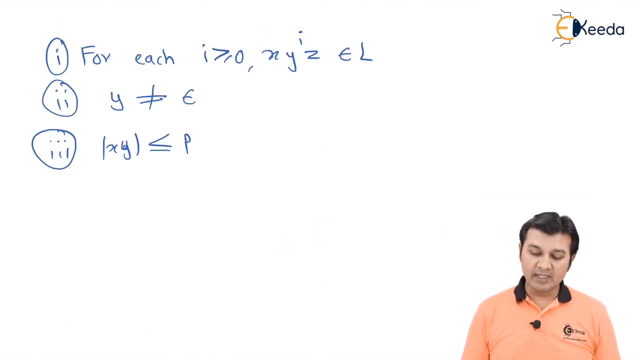 what are the conditions for each? i greater than equal to zero. my x, y raise to y, z to the language. second, my y cannot be equal to epsilon, so pumping length has to consist of some input. it cannot be equal to empty string. lastly, mod of x, y has to be less than equal to the pumping.